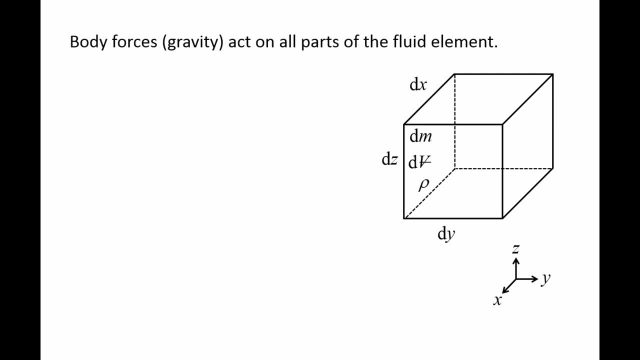 Body forces, such as gravity, act on all parts of the fluid element. The resultant gravitational force acts at the center of mass and points downward. Since the fluid element is very small, we will call this force dfg. The magnitude of the gravitational force is the mass dm times the gravitational acceleration. 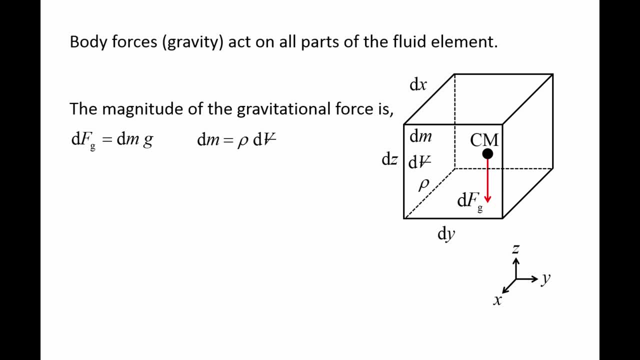 g. The mass dm is equal to the density times the volume. Thank you. There are also forces that act at the surfaces of the fluid element. For clarity, we will only show the forces acting on three of the six surfaces. We can decompose the surface forces into three orthogonal components. 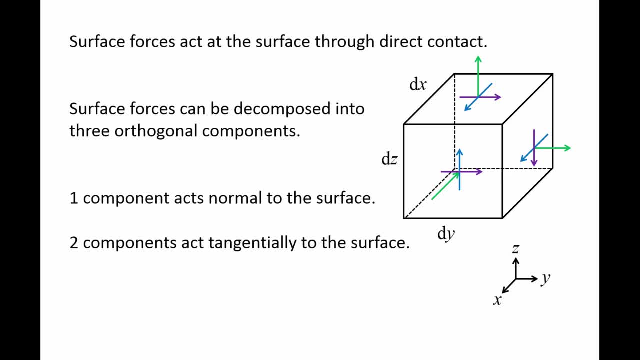 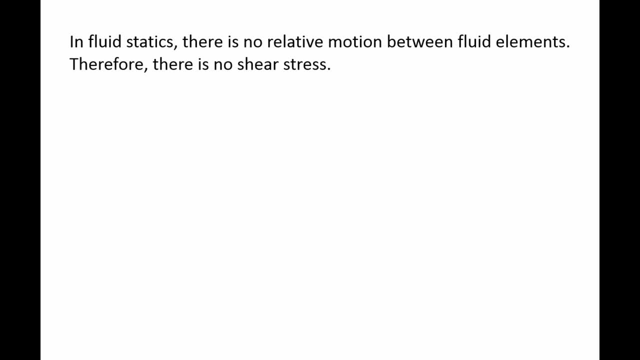 One component acts perpendicular or normal to the surface and two components act tangentially to the surface. There are many systems in fluid mechanics where there is no relative motion between different fluids. For example, the fluid elements do not slide against each other and the fluid would appear. 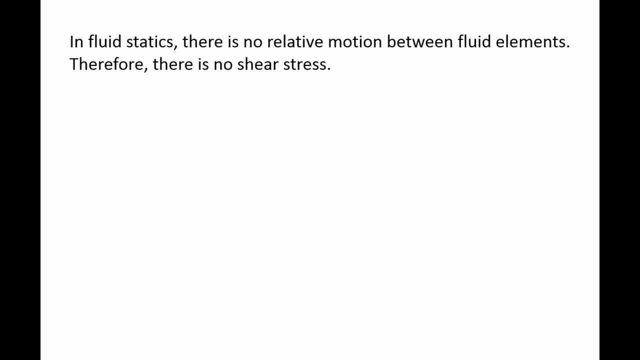 static. Since there is no sliding motion at the surface of the fluid elements, there will be no shear stresses at those surfaces. This occurs in two situations. In the first situation, the fluid is not accelerating. That is, the fluid is either stationary or moving with constant velocity. 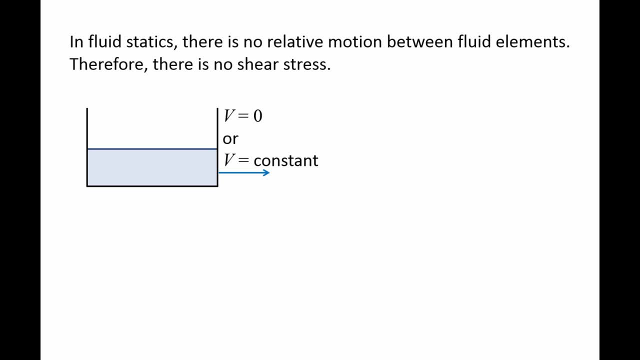 For these systems, the surface of the fluid would remain horizontal. In the second situation, a fluid moves with constant acceleration. If the tank was initially at rest, sloshing would occur. But once the sloshing dies down, although the surface would not be horizontal, it would. 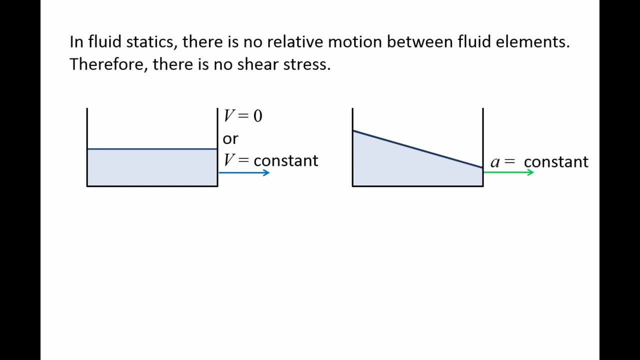 be still and the fluid elements would not slide against each other. In both these situations, a fluid element only experiences normal forces at the surface due to pressure and a gravitational body force. Thank you, Thank you. Since pressure forces act on all sides of a fluid element, we need to know if pressure 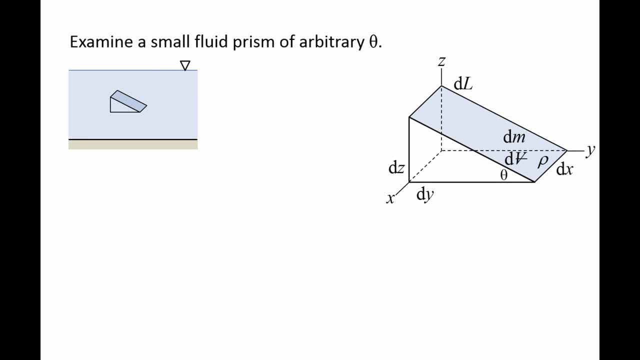 varies with direction. We start by examining the forces on a small triangular prism of fluid of arbitrary angle, theta. The dimensions of the prism are dy, by dz, by dl. The prism has a mass dm and a volume dv and we will assume the density is a uniform. 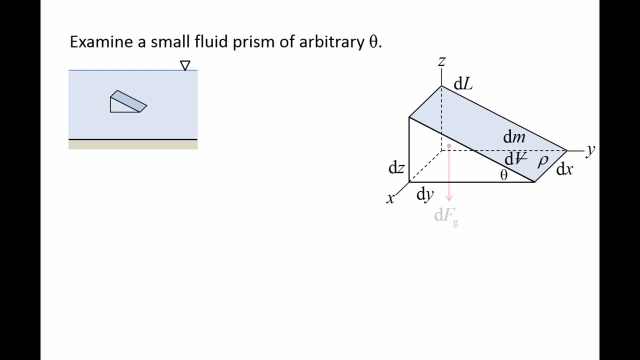 value of rho throughout the prism. The gravitational force dfg acts in the negative z direction And pressure forces act normal to the surfaces. df1 acts on the left side, df2 acts on the top side and df3 acts on the bottom side. 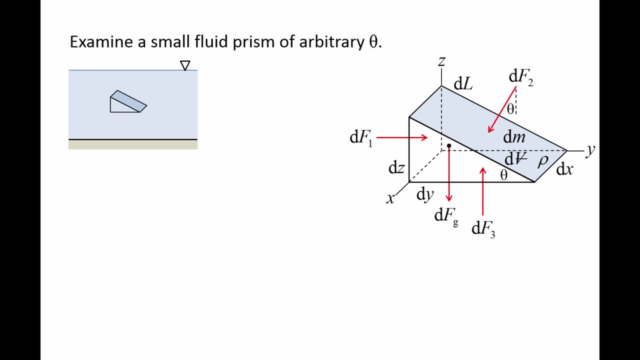 There are pressure forces acting on the front and back sides as well, but including them in the diagram would clutter the image and we would obtain the exact same results whether or not we included them in the analysis. So we omit the forces on the left side. 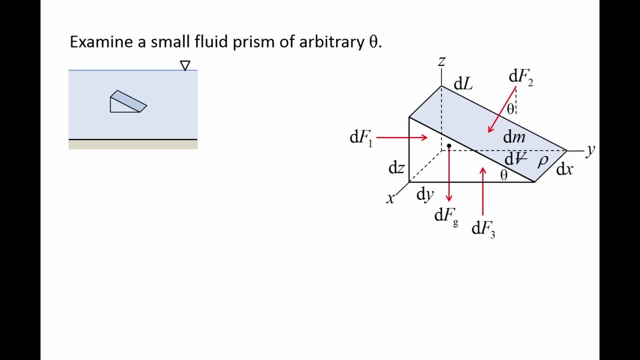 So we omit the forces on the right side, So we omit the forces on the front and back sides. for clarity, Since pressure is equal to force per area, we can rewrite df as pressure times da. So df1 becomes p1 times the area dx times dz. df2 becomes p2 times the area dx times. 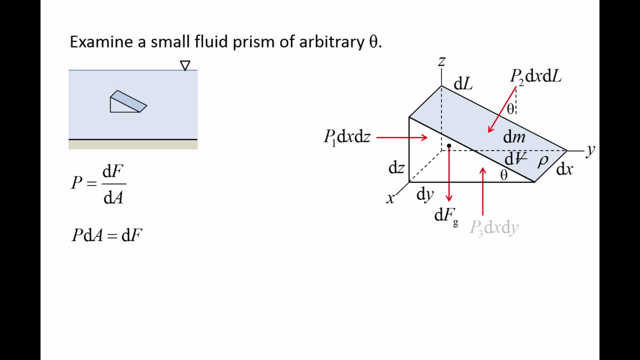 dl and df3 becomes p3 times the area dx times dy. So df1 becomes p2 times the area dx times dl and df3 becomes p3 times the area dx times dy. So df1 becomes p2 times the area dx times dl and df3 becomes p3 times dl. 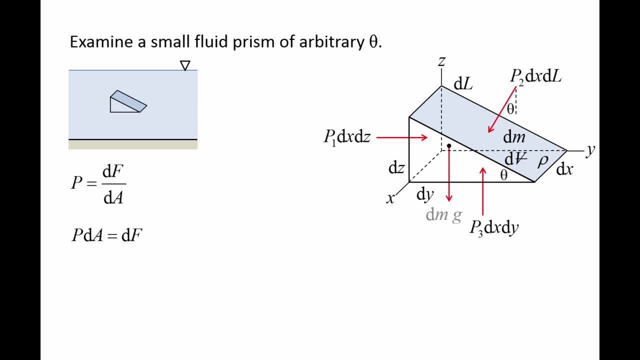 So df1 becomes p2 times the area dx times dl and df3 becomes p3 times dl. We also can rewrite dfg as dm times g. Newton's second law in the y direction states that the sum of the forces in the y direction 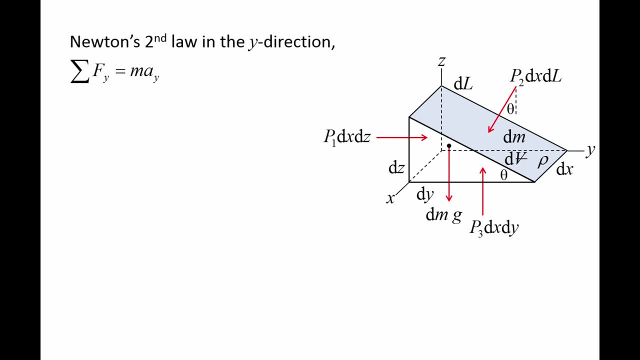 is equal to the mass of the fluid element times the acceleration of the fluid element in the y direction. Substituting the values for forces and mass, we get p1 times dx dz minus the y component of the pressure force. on the top, This is the p2 times dx times dl, sine theta, which equals the dm times ay. 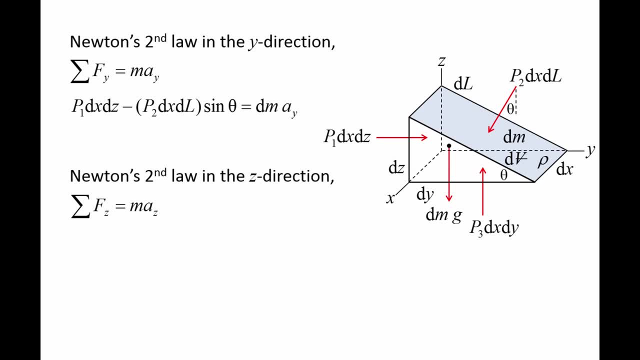 Newton's second law in the z direction states that the sum of forces in the z direction is equal to the mass of the fluid element times the acceleration of the fluid element in the z direction. Substituting the values for forces and the mass, we get p3 times dx, dy minus the z component. 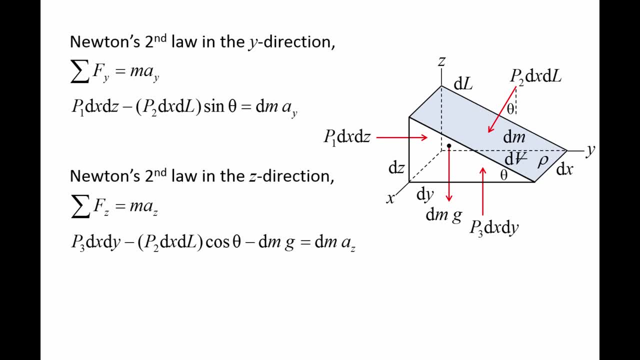 z component of the pressure force on the top face: P2 times dx, dl cosine, theta minus dm times g equals dm times az. For this analysis we will not apply Newton's second law in the x direction as the symmetric.